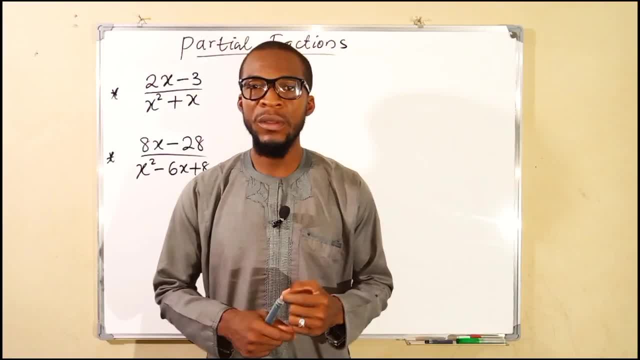 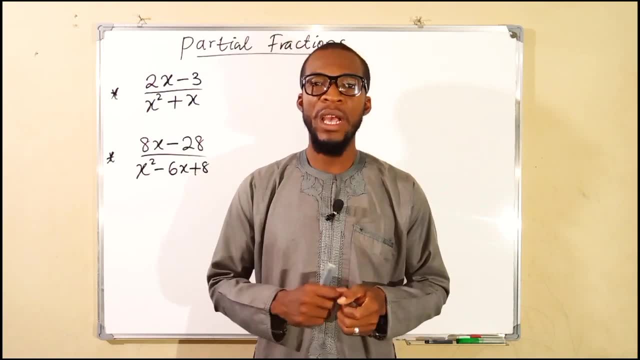 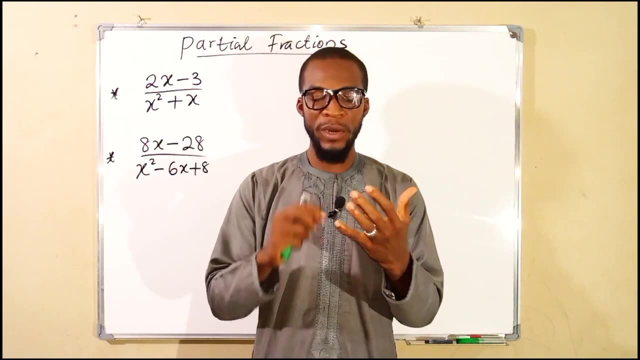 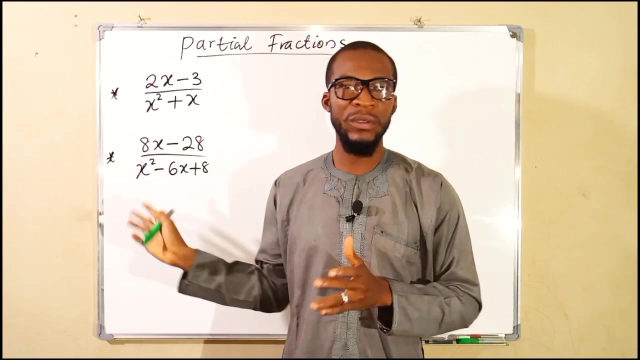 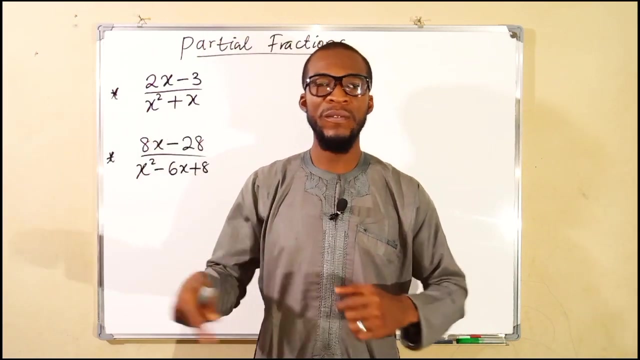 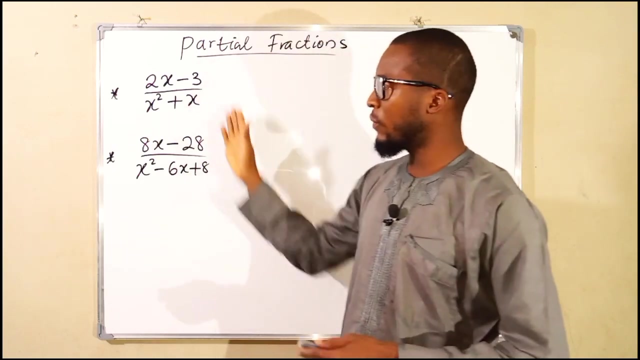 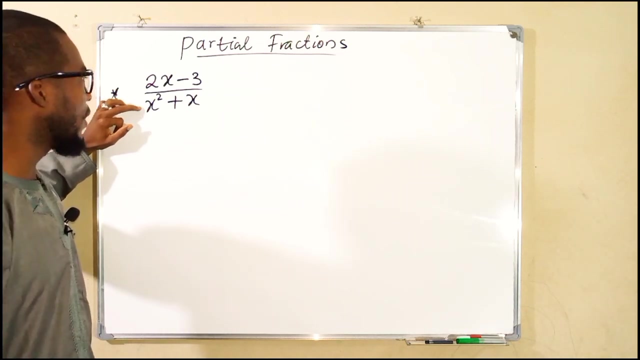 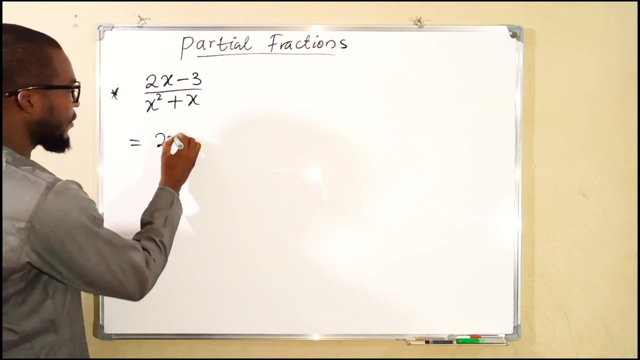 Hello good day viewers. This is the continuation of our lesson on how to split compound fractions into partial fractions. Throughout in this topic I shall only be discussing based on three components of fractions. The first one is when we have repeated factors under the denominator. The second one when we have no repeated factors and the last one is when we have the degree of denominator greater or equal to the degree of the denominator. So I have two problems here which I want to resolve for today. Let us start with the first one. This is a fraction but if you look at the denominator it is not written in factored form. Hence you have to factorize it first. So we can write this as 2x minus 3 divided by. You can see we have X in bottom. 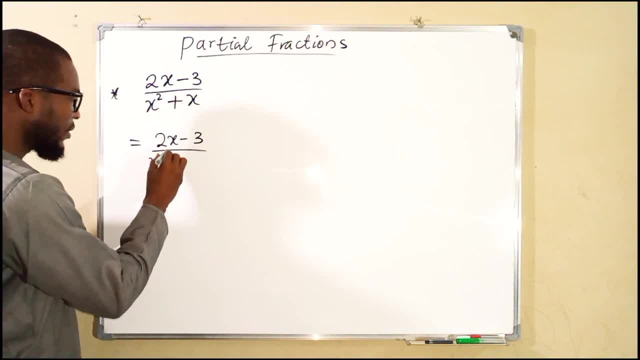 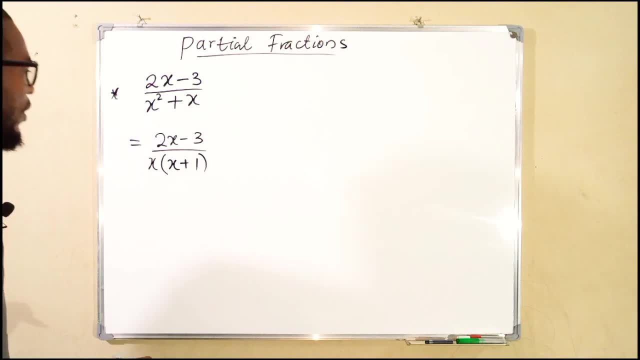 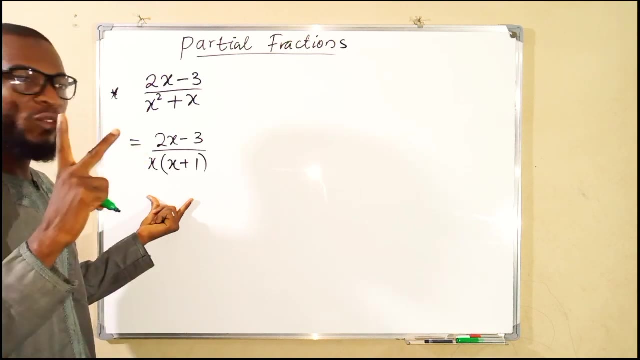 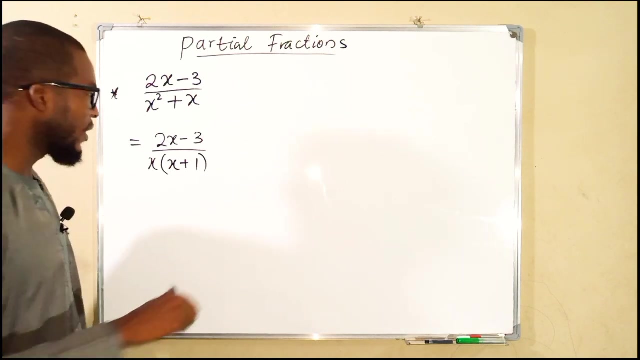 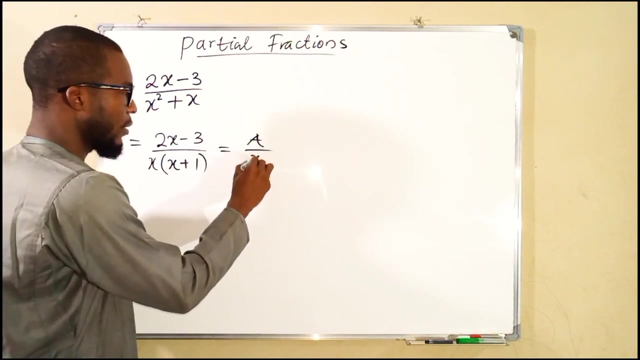 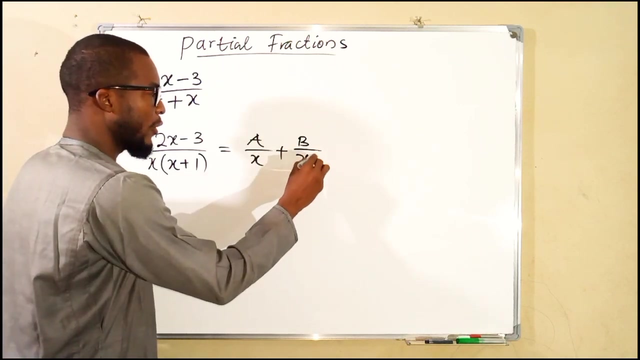 So we can write this as 2x minus 3 divided by. You can see we have X in bottom. So we can write this as 2x minus 3 divided by. You can see we have X in bottom. of this two times so we can factor X out and inside we have X then plus 1. This is our factorized form of fraction and you can see we only have two factors and hence we are going to obtain only two fractions and each of these factors are linear factors and therefore their corresponding numerators are going to be constants. So this is equal to a over the first factor which which is x, then plus another constant b over the second factor x plus one. If we apply cover-up method, 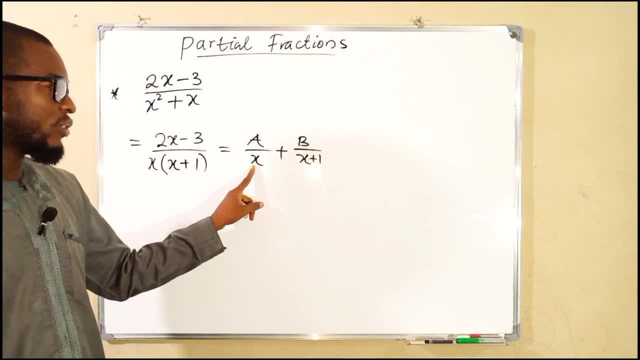 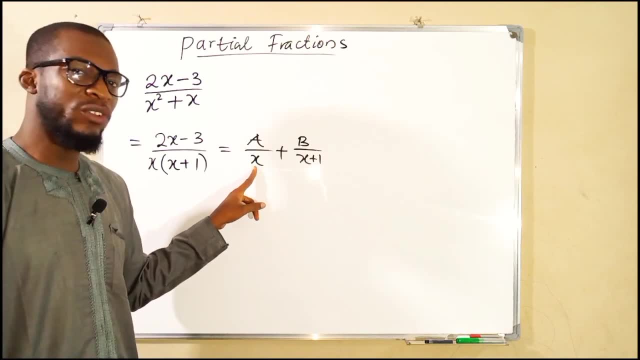 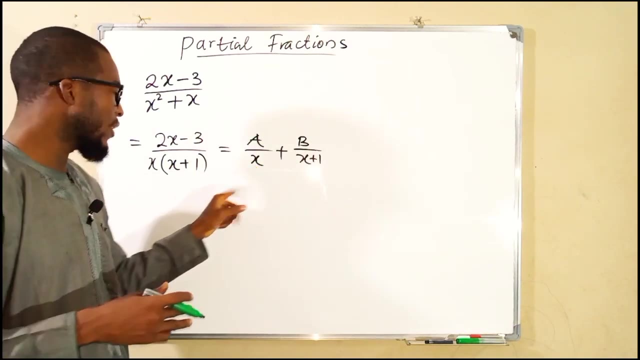 we are going to start with the first one. We are going to think of the way to transform this denominator into zero, and it can only be done by setting the value of x to be equal to zero. So if x is zero, the denominator is going to be zero, and we are going to substitute that zero into the other factor. 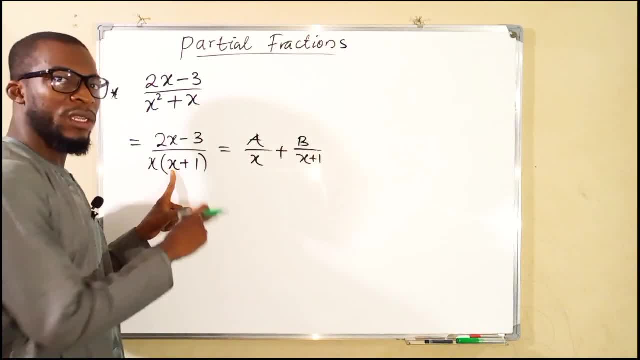 We can see if we substitute zero here, we have zero plus one is equal to one, and we have one x, which can also be written as x. 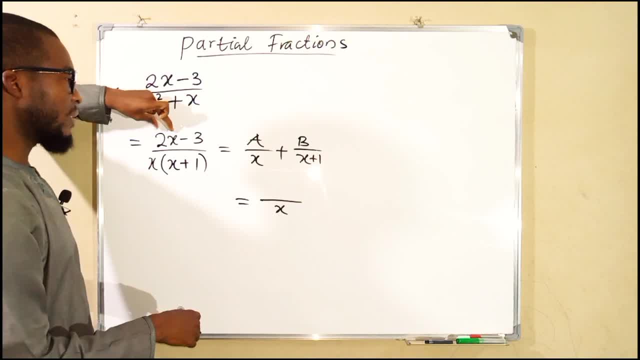 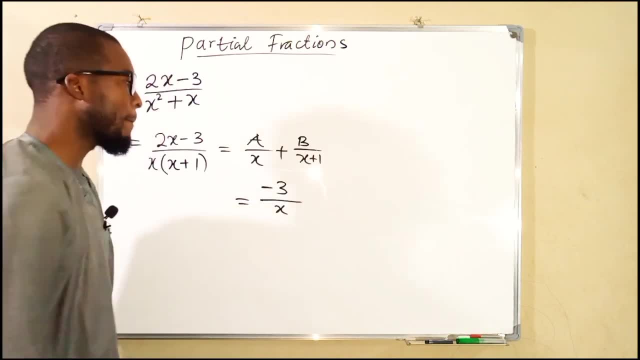 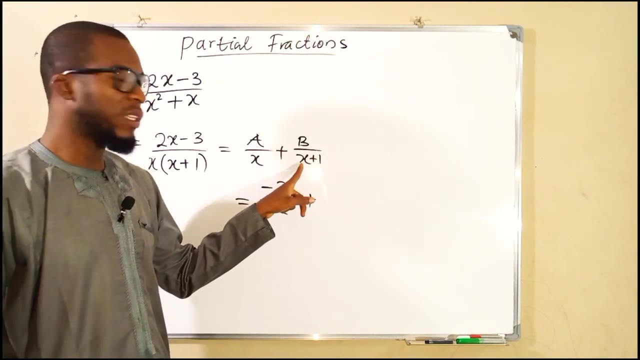 Then to the top, we substitute zero to the top. You can see zero times two is zero. Minus three is minus three. So we have minus three to the top, minus three. Then plus, you move to the second one. To transform this into zero, we have to set the value of x to be equal to negative one. 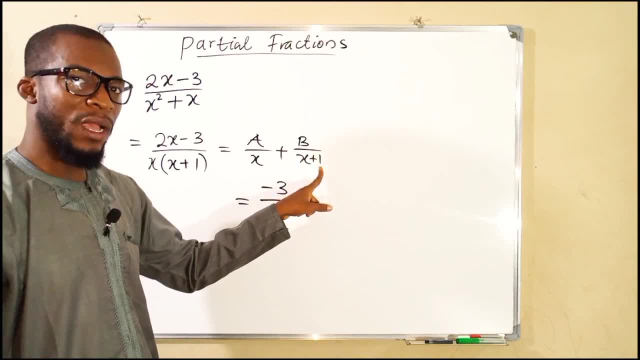 Negative one, positive one, is zero. And that negative one has to be substituted in the other factor, which is x. 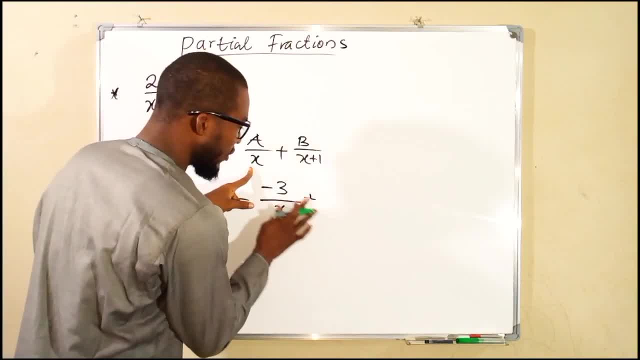 So we have negative one. So this will transform this into negative, our denominator, x plus one. 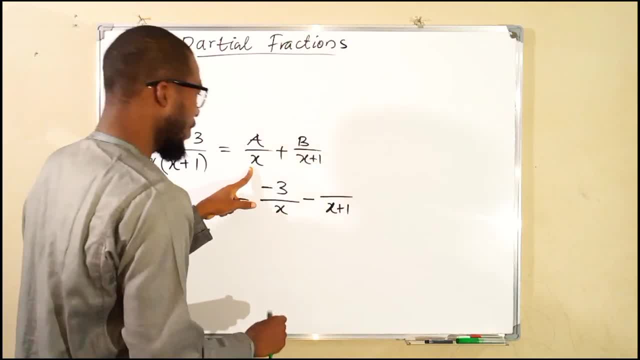 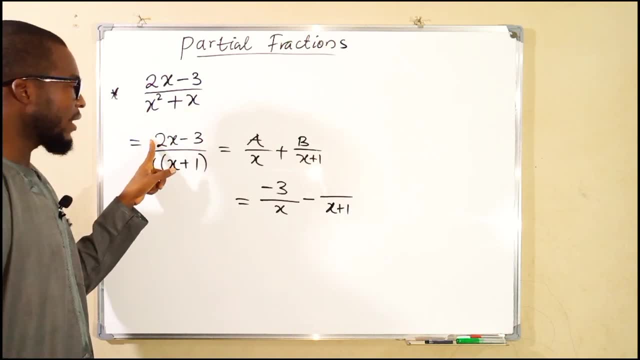 You know that value is one, so it will not affect this then substitute that negative 1 to the top negative 1 times 2 is negative 2 then negative 2 negative 3 is negative 5 so 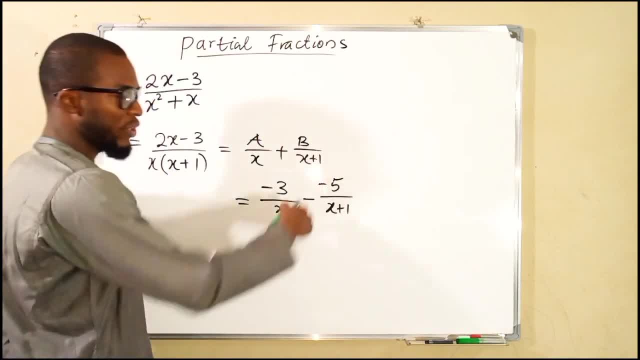 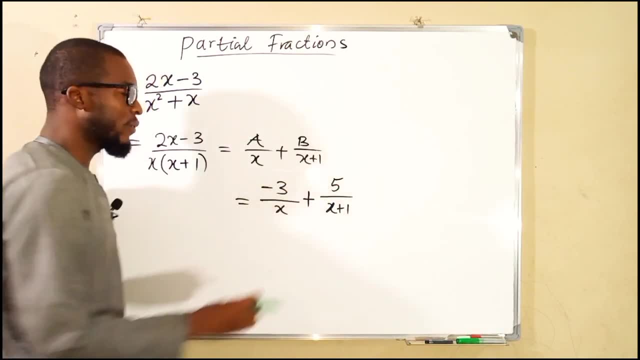 we have negative 5 here which can also be transformed into positive because we have two negatives so this becomes positive and hence this is our partial 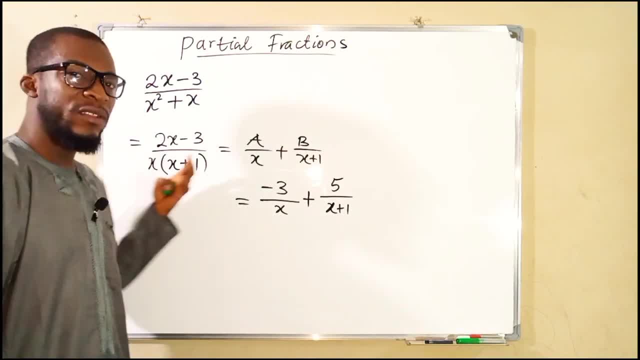 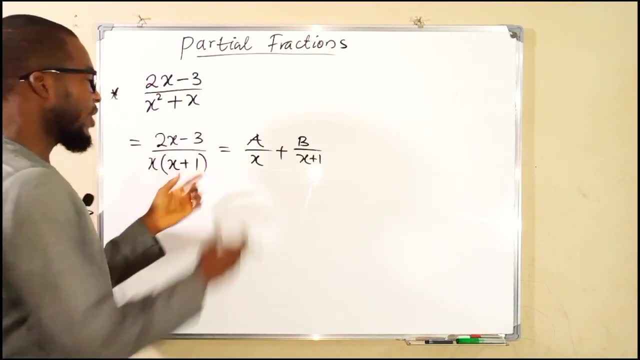 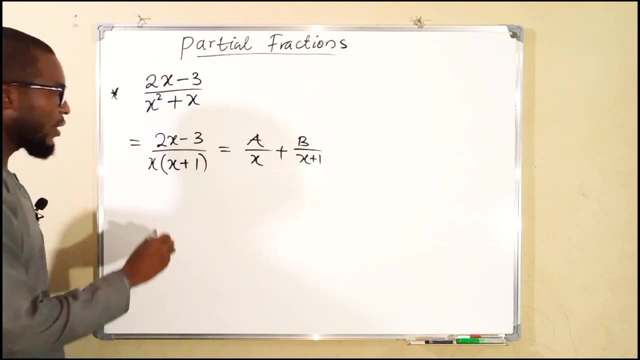 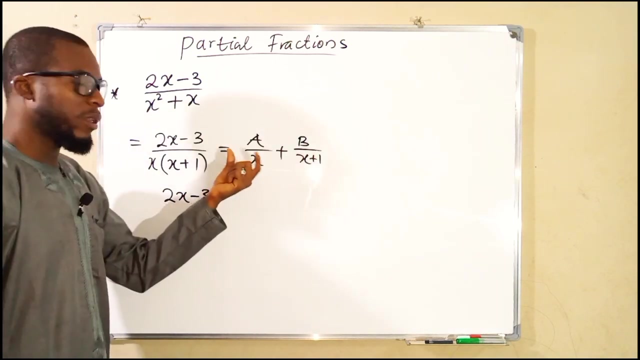 fraction of this compound fraction and this is not the only way to find this constant let me show you the other way the other way is by multiplying each time by the factors under the denominator here so multiply this side by X times X plus 1 you will be only left with 2x minus minus 3 and if you multiply this 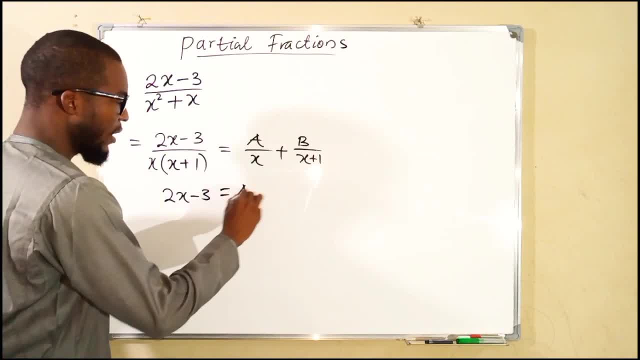 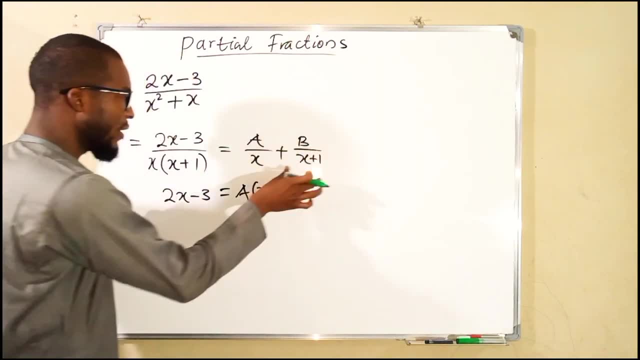 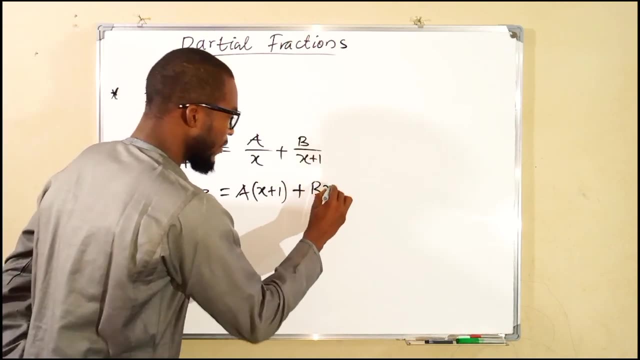 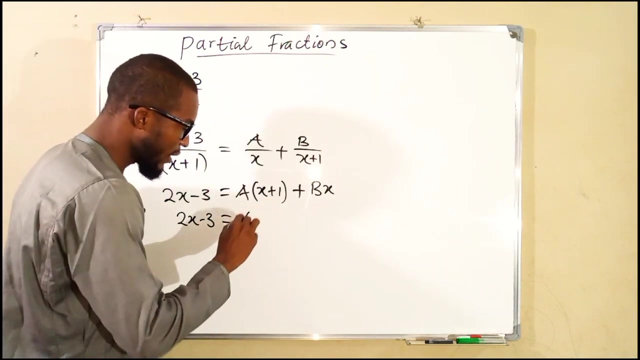 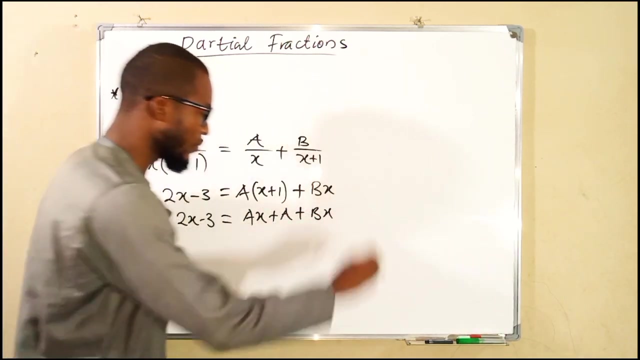 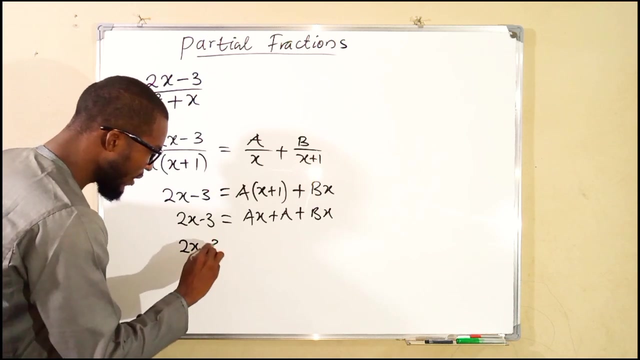 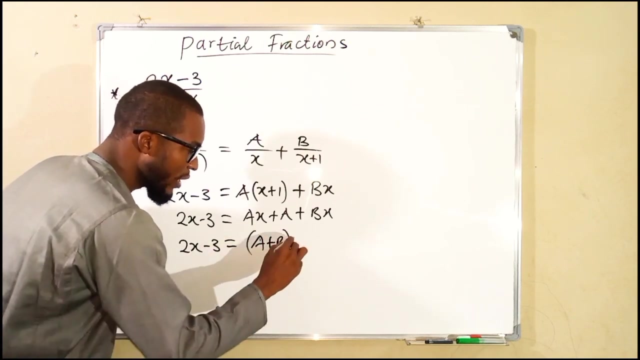 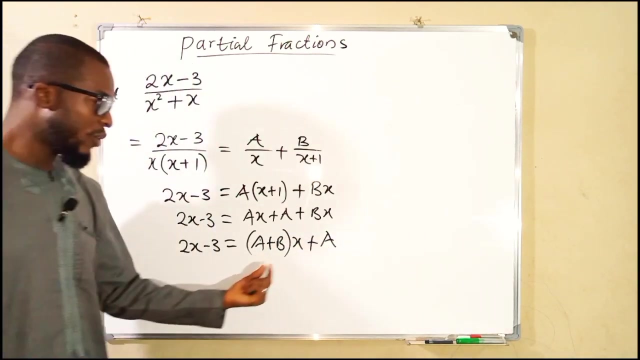 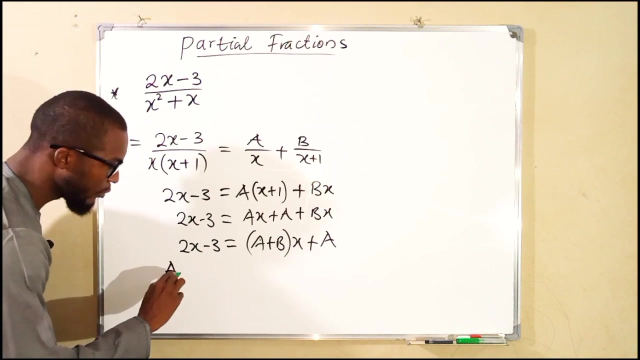 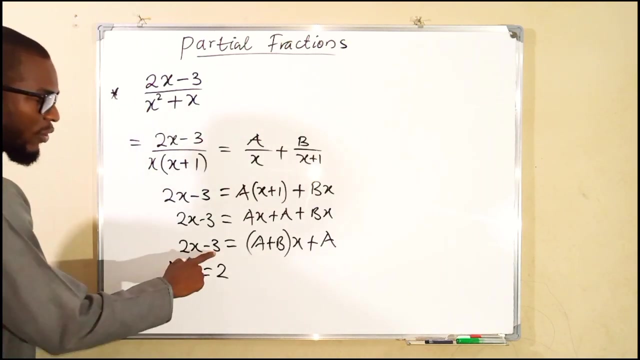 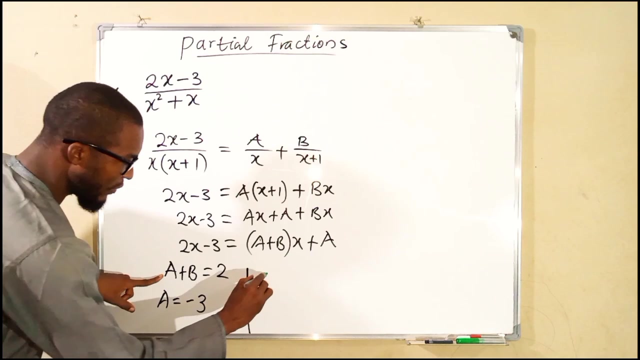 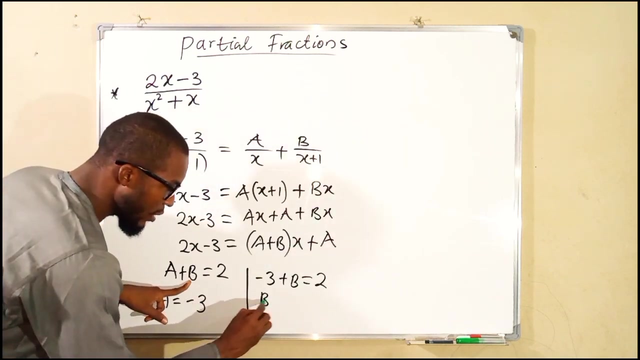 by these factors you are going to obtain a a a ,x plus 1 because this X will cancel this other X then plus multiply this by these two factors this X plus 1 will cancel this leaving only this so we have only bx 2x minus 3 will be equal to if you expand this you obtain ax plus a plus bx again let us bring those with X together so we have 2x minus 3 this is equal to you can factorize it as a plus B when you bring X out then plus our a so by relating the coefficients you can see the coefficient of X to the right is a plus B while the coefficient of X to the left is just 2 so we have a plus B equals 2 while a is equal to the constant which is negative 3 so we have a equals negative 3 if a is negative 3 you can substitute it back here so we have instead of a we have negative 3 then plus B this is equal to 2 to find B you take negative 3 to the right we have 2 plus 3 and B equals 2. 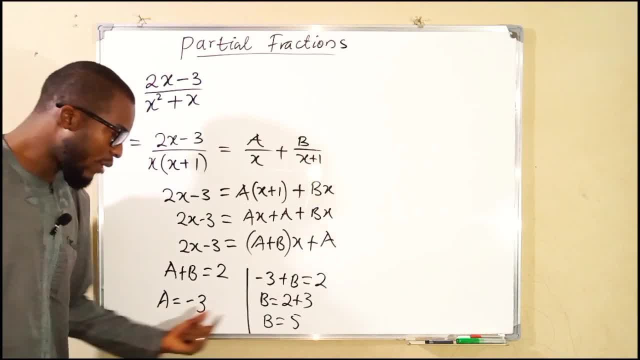 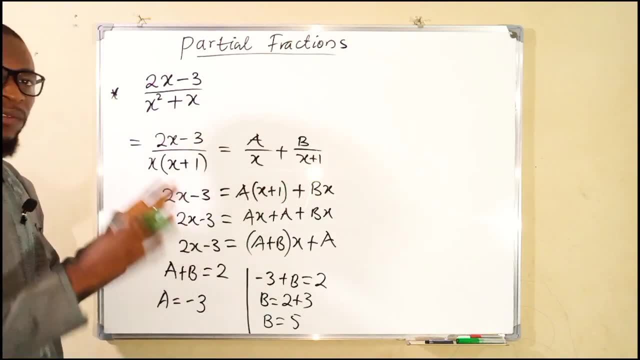 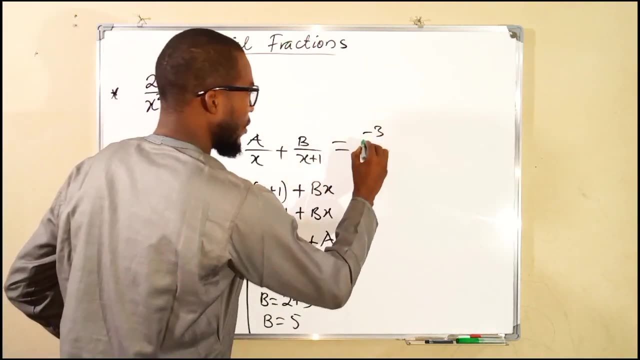 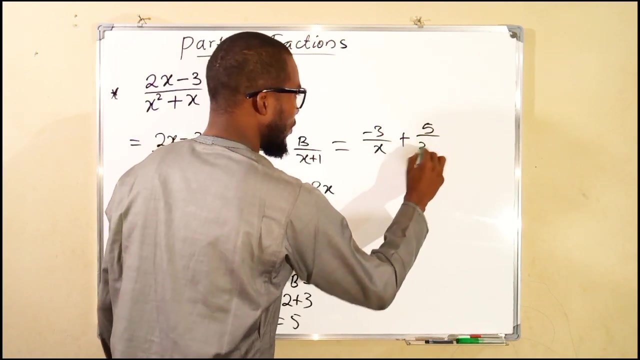 because 5 and therefore the values of a and B are negative 3 and positive 5 respectively and you can substitute them back into this expression to obtain the partial fraction of this compound fraction so we can write this one as our a you can see it as negative 3 over the first factor X then plus our B is 5 over the second factor which is X plus 1 and this is our partial fraction of this compound fraction 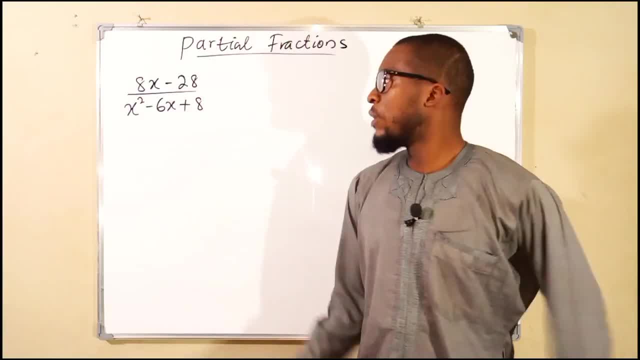 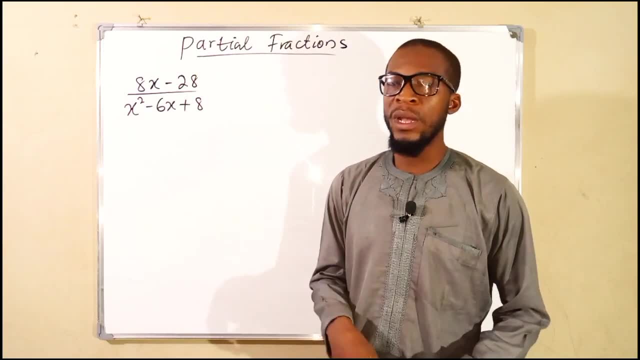 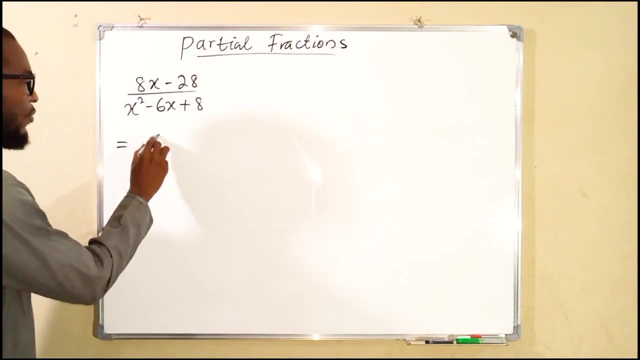 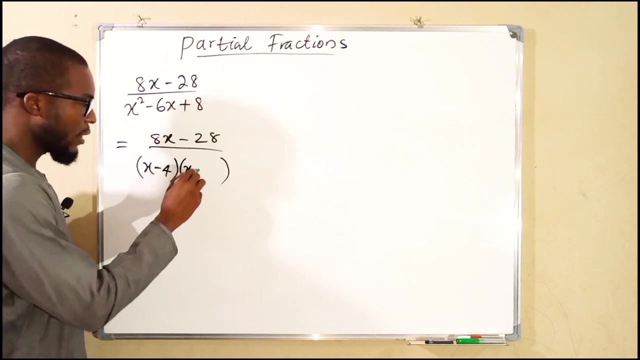 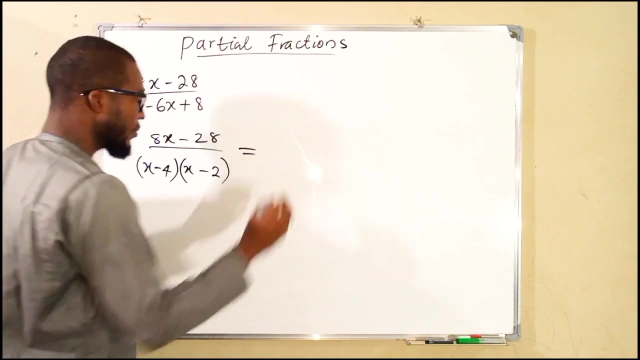 so now let us look on to the last example so here is our next example you can see the denominator is not written in factored form and hence we have to factorize this quadratic function to factorize it we have this is equal to 8x minus 28 over we're going to obtain two factors we're going to think of two numbers which when we multiply them together we get positive 8 and when added up together we get negative 6 and the numbers are negative 4 and negative 2 because negative 4 times negative 2 is positive 8 negative 4 negative 2 is negative 6 so this is what we have to resolve to partial fractions all of them are linear factors therefore their 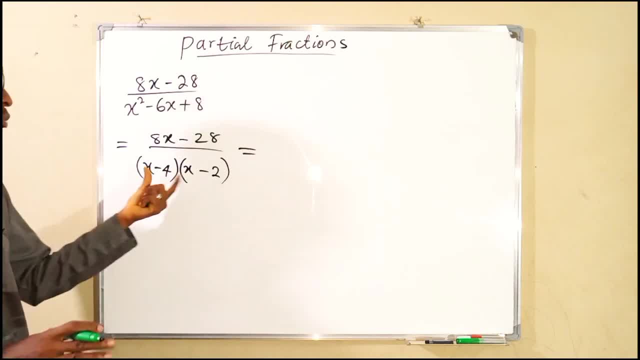 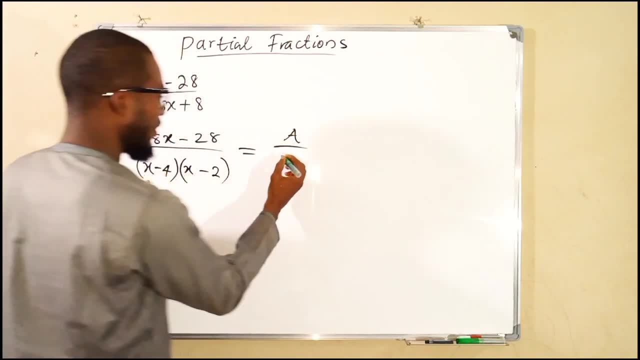 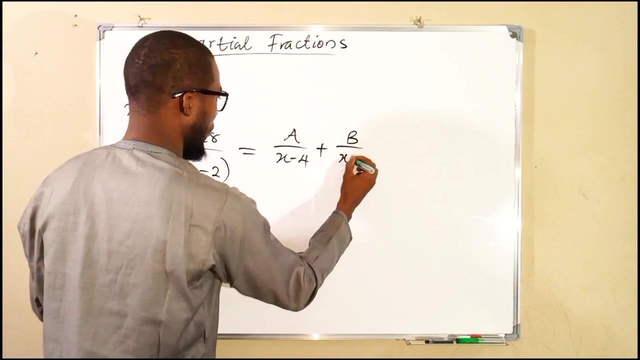 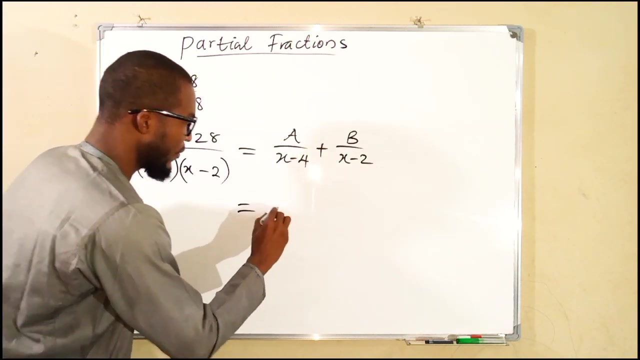 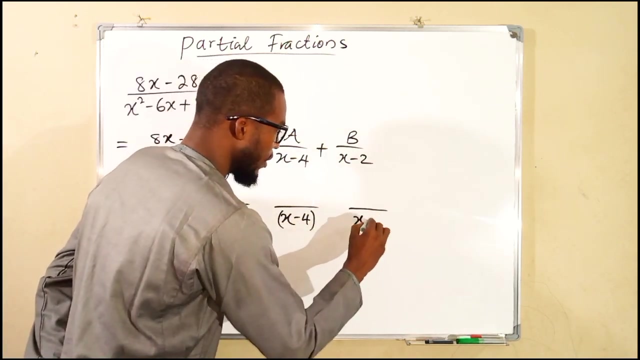 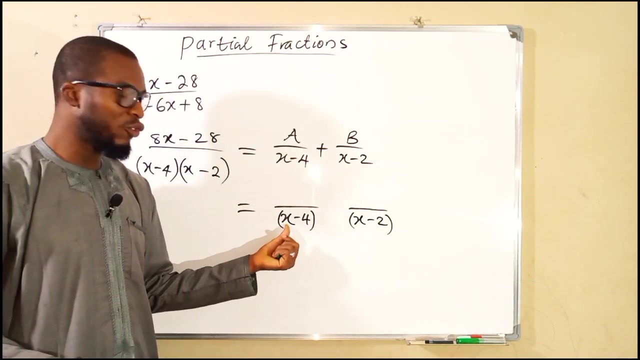 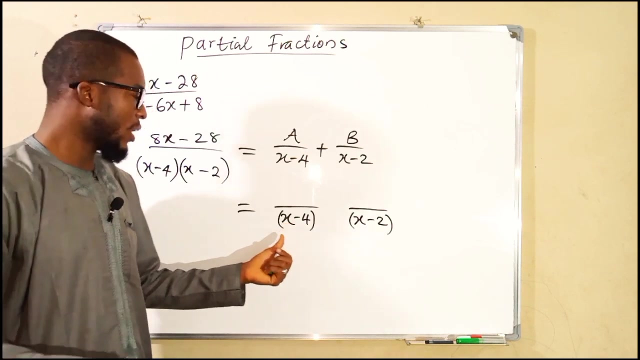 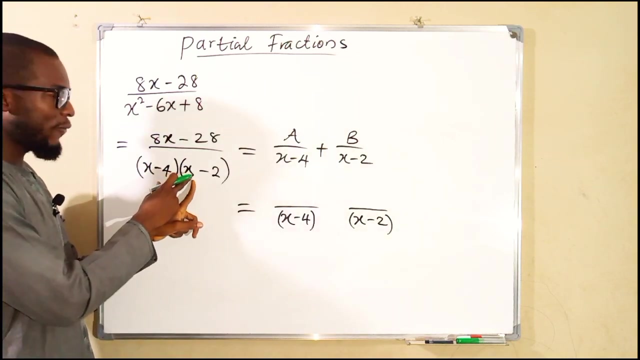 corresponding numerators are going to be constants and also denominators where positive is not negative so taking this one when I'm just because there are two factors we're going to obtain only two fractions so the first one is going to be a over the first factor X minus 4 then plus another constant over X minus 2 let us start solving this by cover up method we have our first fraction Let us first of all consider this, to transform this into zero, x must be equal to four. Four minus four is zero, and we are going to substitute that four into the other factor. If x is four here, four minus two is two, so we have our two here. 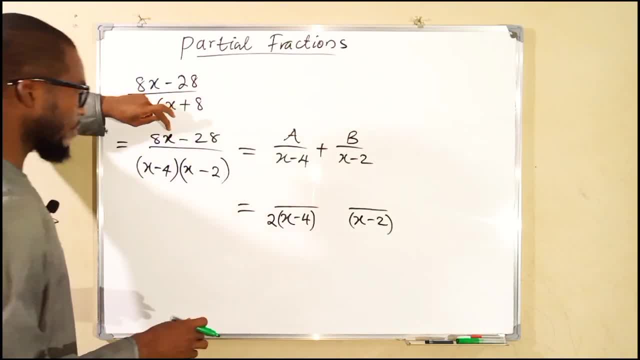 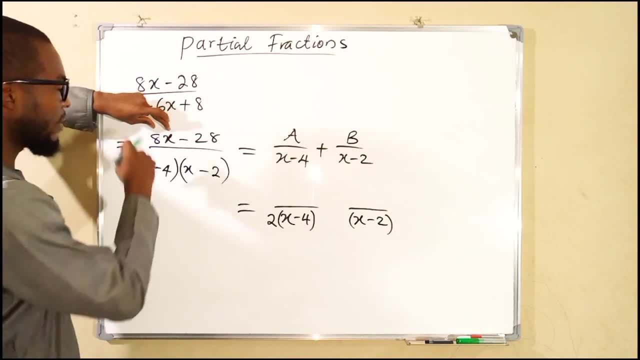 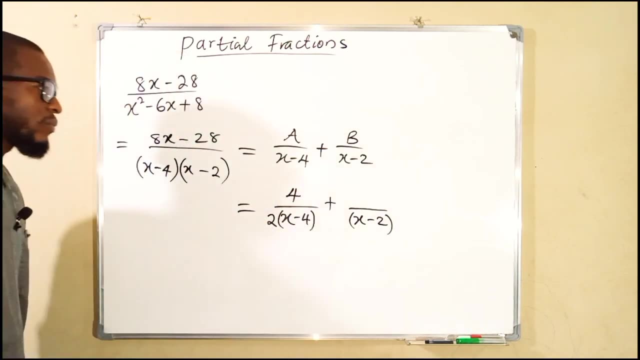 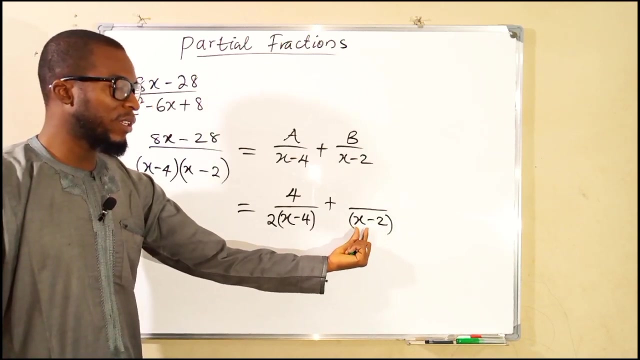 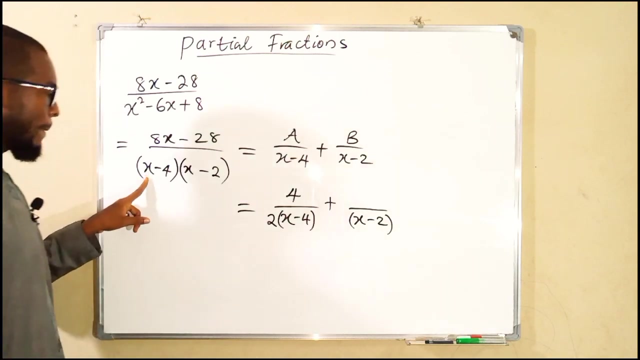 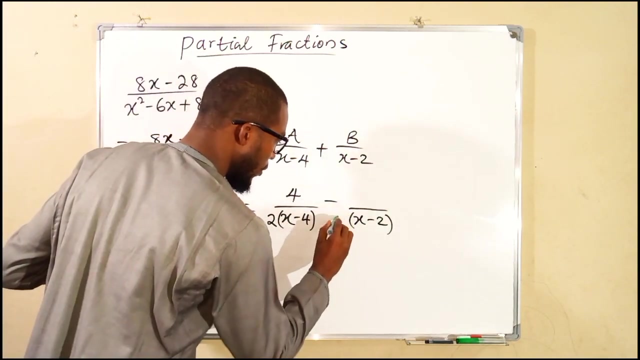 Then to obtain the top number, we are going to substitute that four here. You can see four times eight is thirty-two, then thirty-two minus twenty-eight is four, so we have four here, plus. The other factor is x minus two. To make it zero, we have to set the value of x to be two, so that two minus two is zero. That two is going to be substituted here. We have two minus four. It's minus two, so instead of plus here, we have minus two. 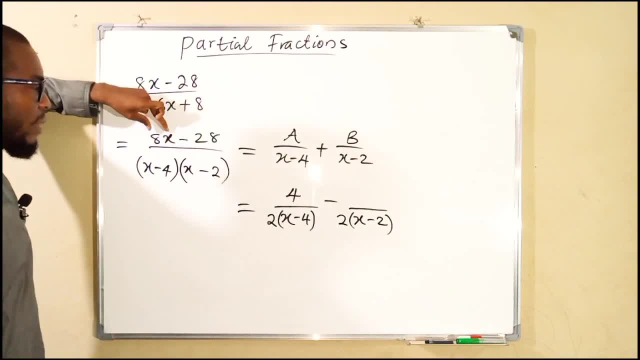 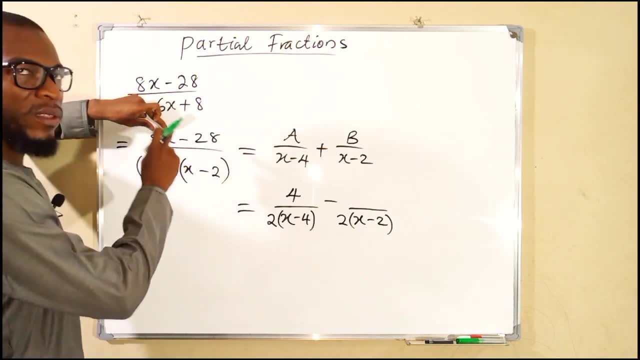 Then to the top, we have two times eight is sixteen, then sixteen minus twenty-eight is minus twelve. 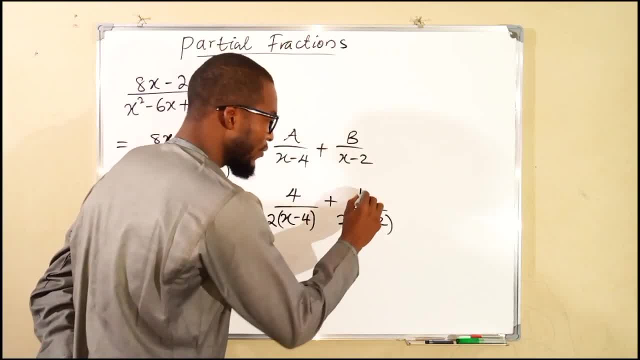 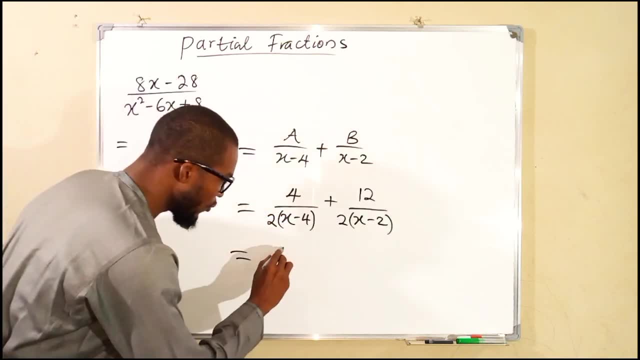 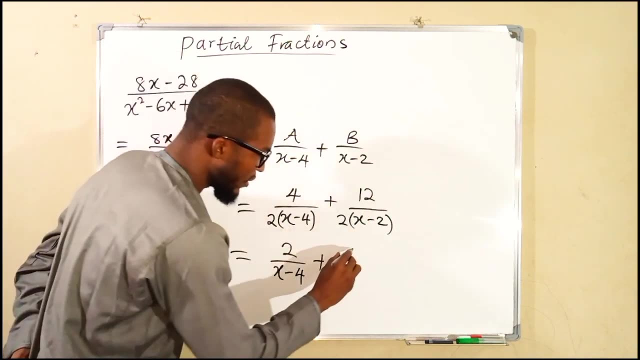 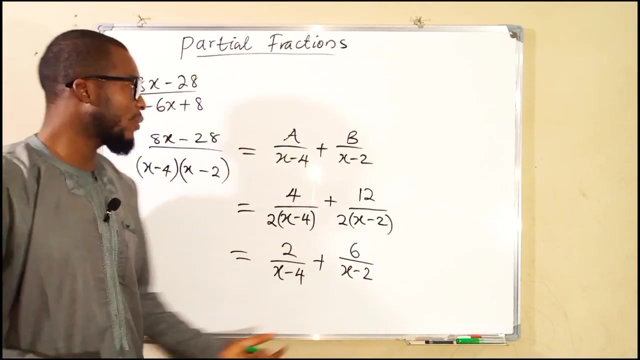 So we have, this becomes positive, and we have twelve here. This can also be reduced into, because two can go into four two times, so we have two. Over x minus four, then plus two can go into twelve six times, so we have six over x minus two. And these are the partial fractions of this compound fraction. 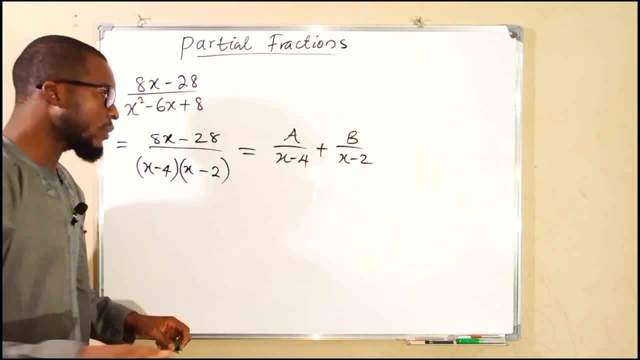 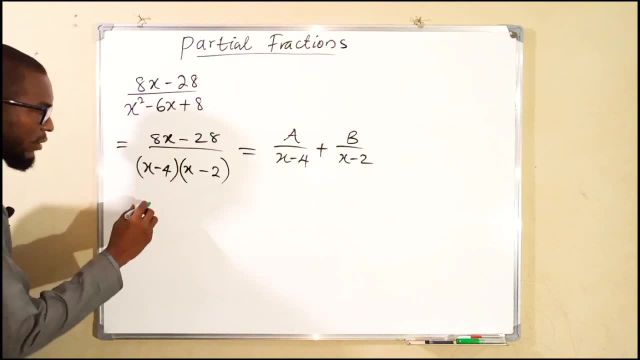 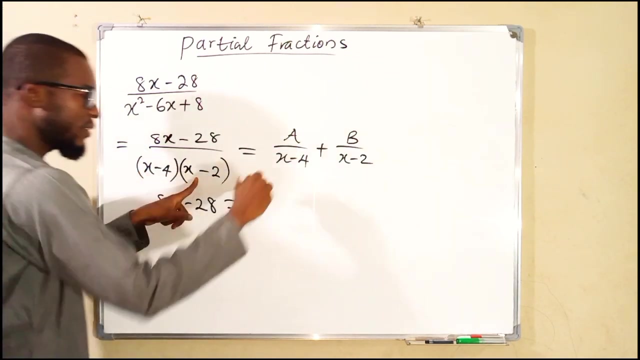 Let me show you the second method. We are going to multiply each of these times by these two factors. The first one, if after multiplying by these two factors, they are going to clear up, leaving only the numerator. At x minus twenty-eight, and this is equal to this multiplied by this, this will be taking care of this, leaving only this. So we have a x minus two, then plus the other one. 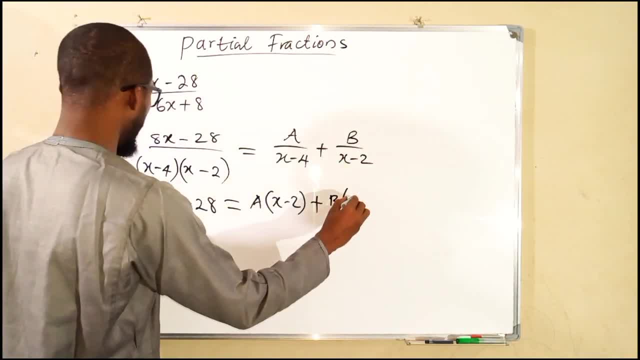 This will cancel this, leaving this, so we have b multiplied by x minus four. 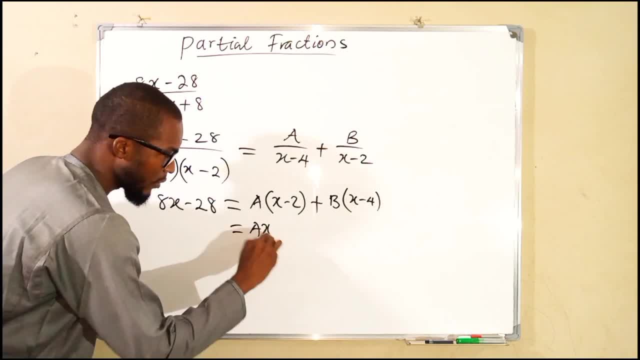 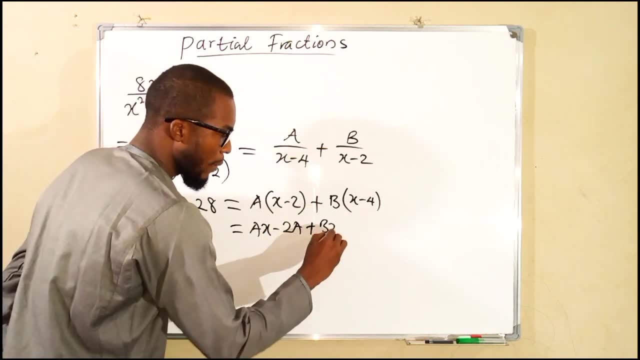 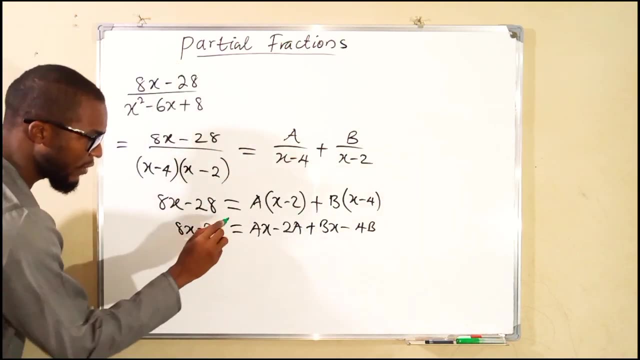 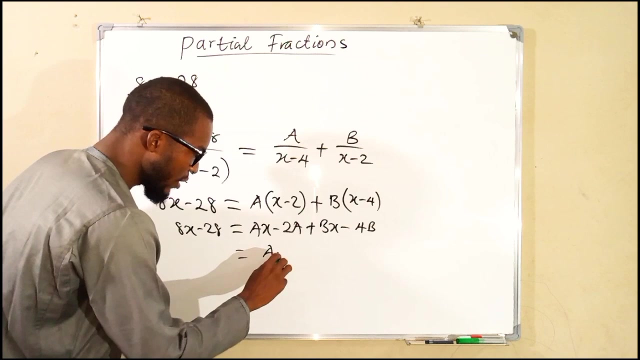 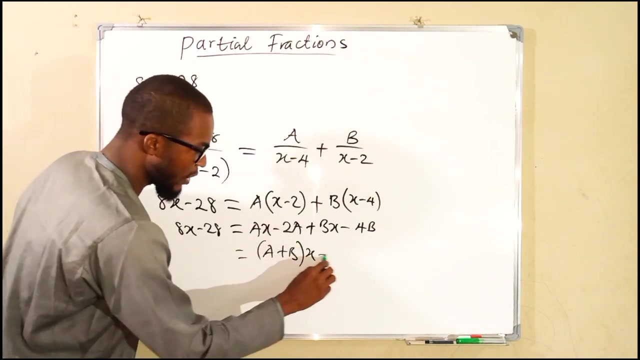 Let us expand them. This is equal to a x minus two a plus b x, then minus four b. This is eight x minus twenty-eight. Let us bring those with x together. We can equally factorize them. So we have a plus b, this and this, all multiplied by x. And the constants we have. Minus two a and minus four b. 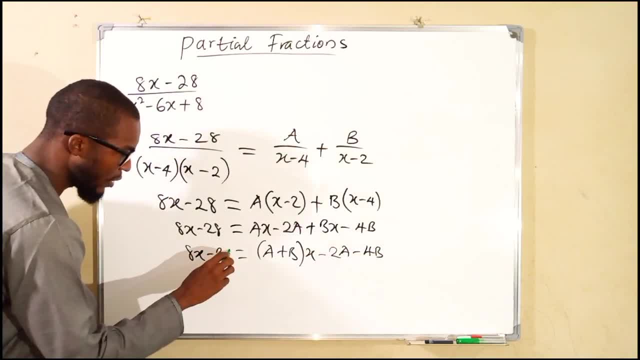 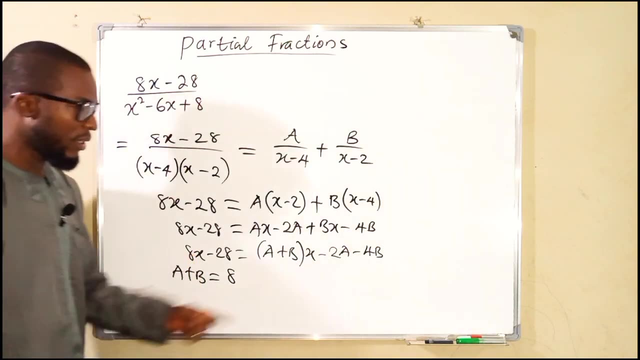 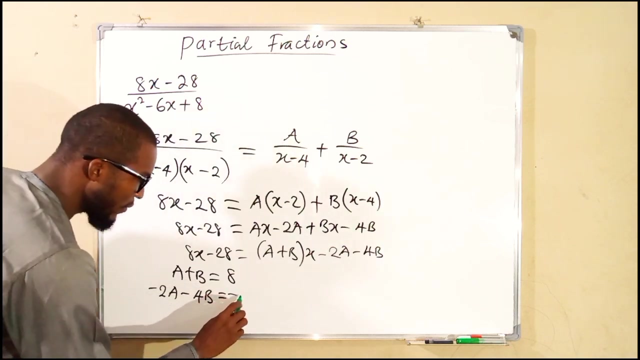 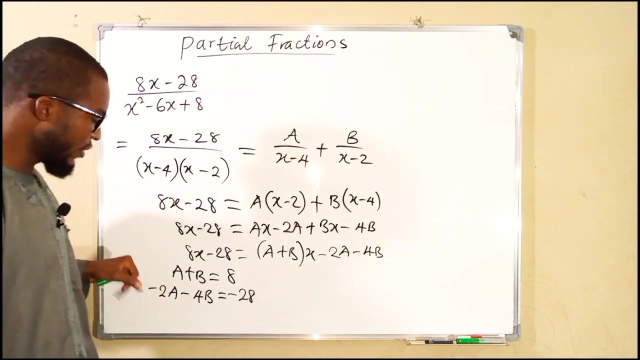 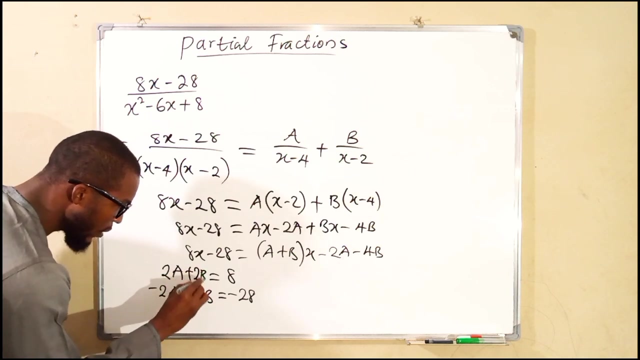 And to the left we have eight x minus twenty-eight. By relating the coefficients, you can see a plus b, a plus b must be equal to eight. The coefficient of x is a plus b, the coefficient of x here is eight. And the constants here we have minus two a. Minus four b is equal to the constant here, negative twenty-eight. We can solve these two equations simultaneously. We can equally multiply this equation by two, so that we can eliminate a. So to do that, you can multiply all of them by two. So here we have two b. 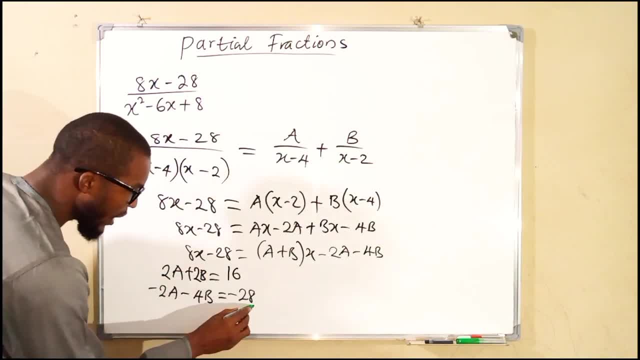 And here we have seven. And here we have sixteen. 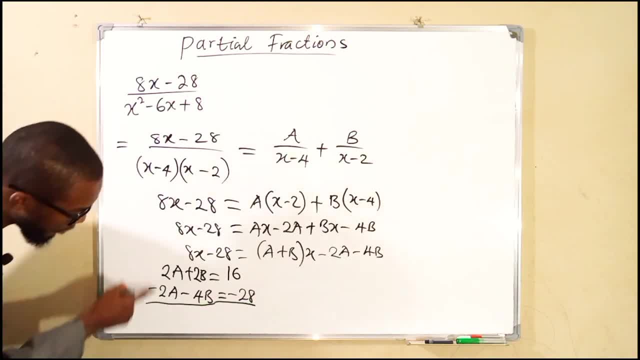 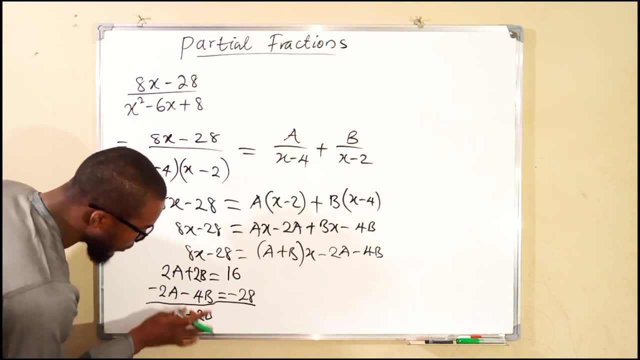 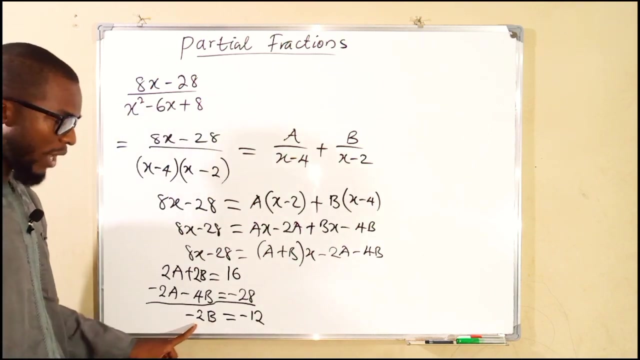 Now we can add these two equations together. This plus this is going to be zero. And this plus this is going to be minus two b. And this is equal to, this plus this is going to be negative twelve. To find the value of b, we divide both sides by negative two. And you can see it here. 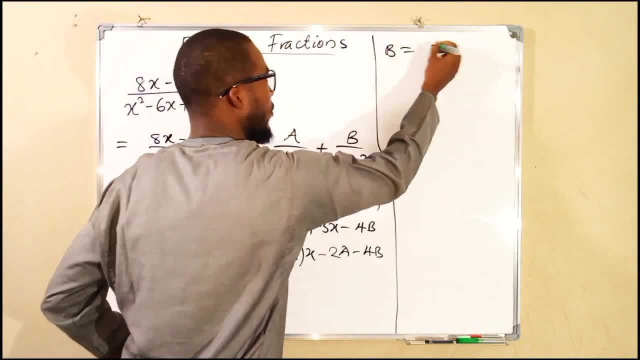 That b will be equal to negative twelve over negative two. 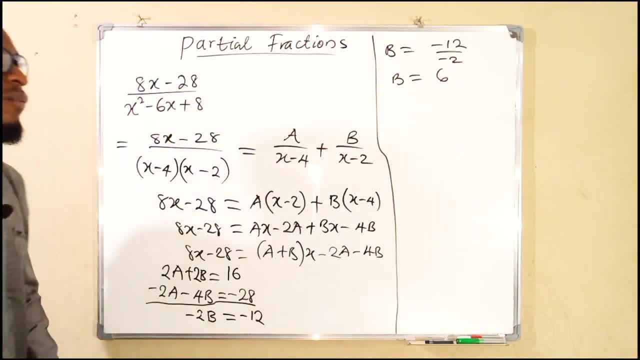 And b is now equal to positive six. Having obtained the value of b to be equal to six, we can substitute it back into this 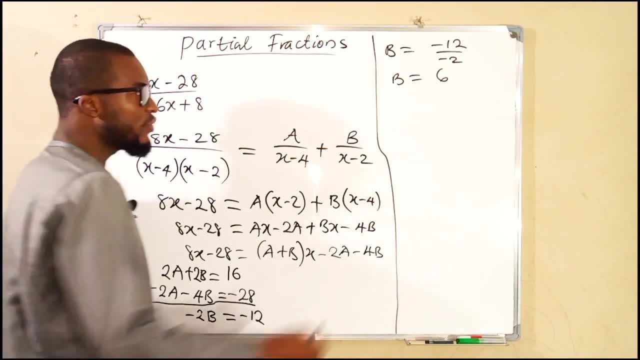 equation, or this equation. 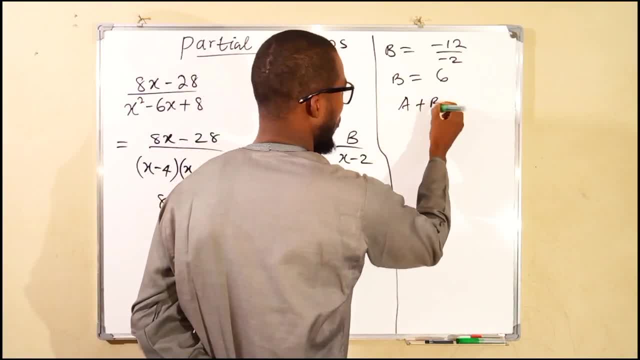 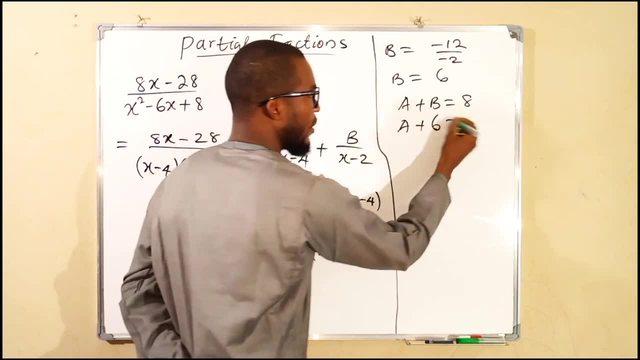 But initially we have a plus b to be equal to eight. This means that a plus b is equal to eight. This means that a plus b is equal to eight. This means that a plus b is equal to eight. This is six now. This is equal to eight. 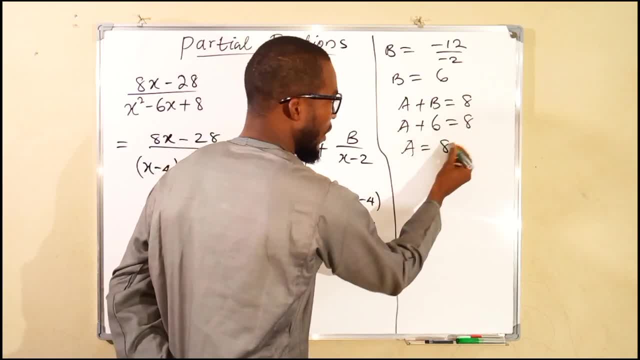 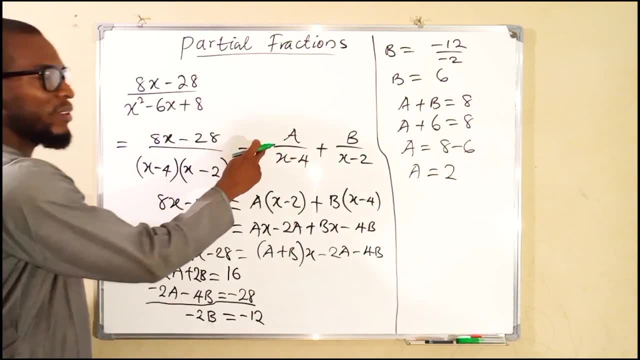 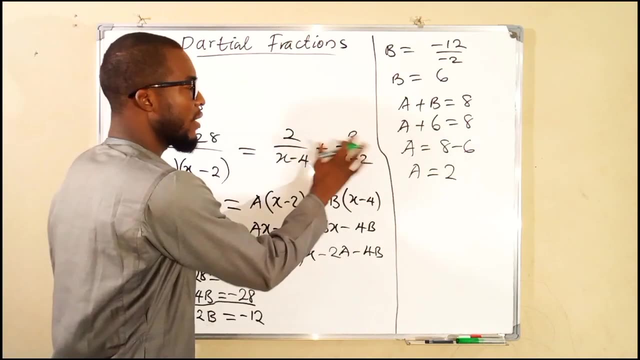 If you take six to the right hand side, we have a equal to eight minus six. And a now will be equal to positive two. We substitute that back into this expression to obtain our partial fractions. You can see a is equal to two, while b is equal to six. 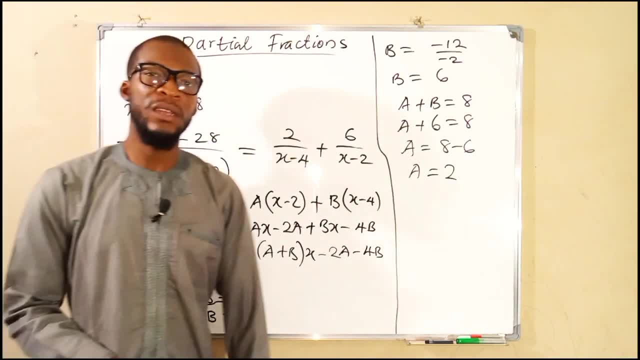 And these are the partial fractions of this compound fraction. 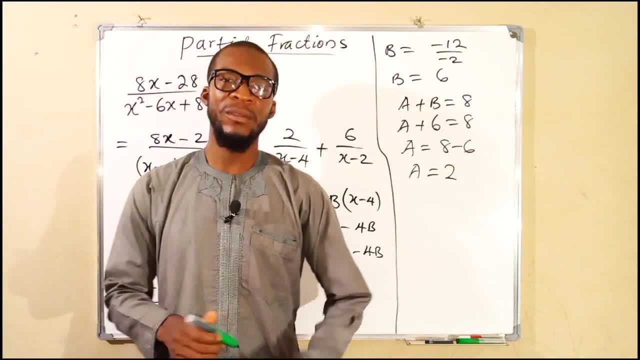 And this is all I have for you today. Thank you for watching. Do have a nice day.